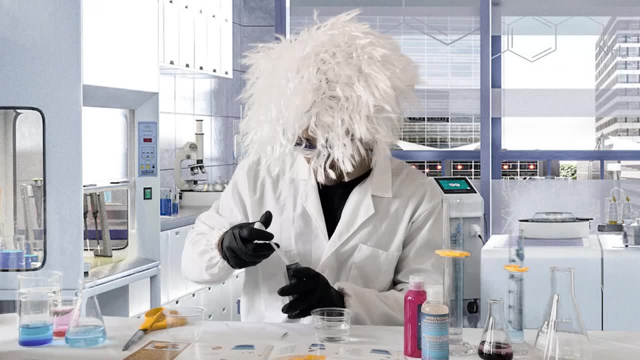 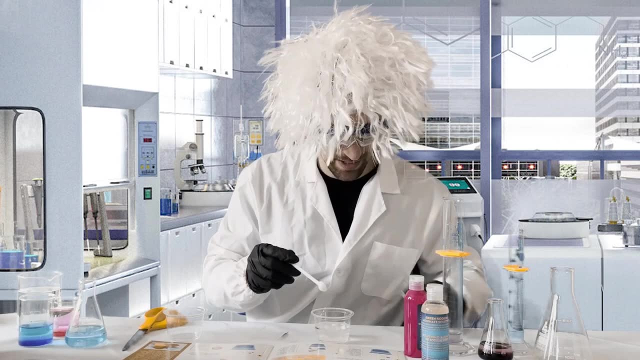 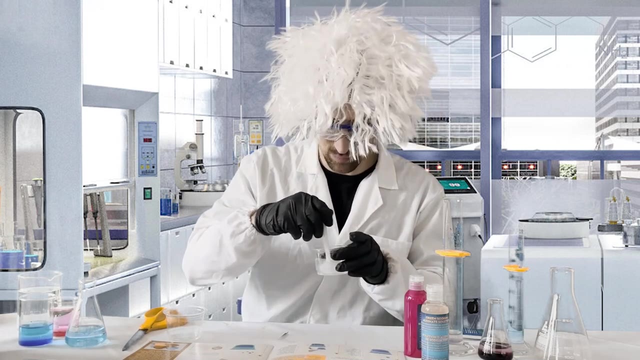 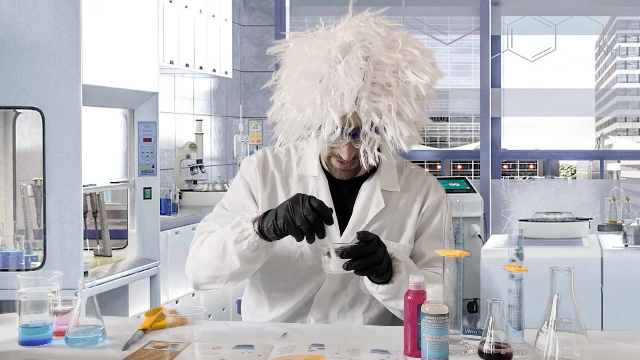 small spoon of calcium chloride. So, just like that, I'm putting in that small spoon of calcium chloride and I'm going to be mixing this until the calcium chloride powder is fully dissolved. That gives us a solution here that's filled with this calcium chloride which we'll see in a moment. 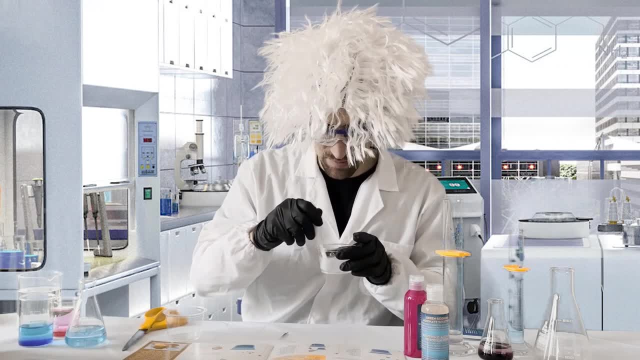 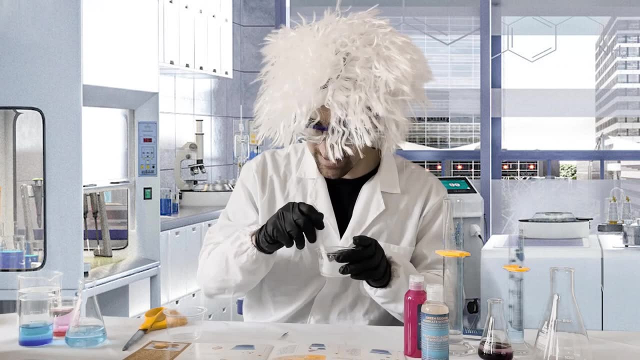 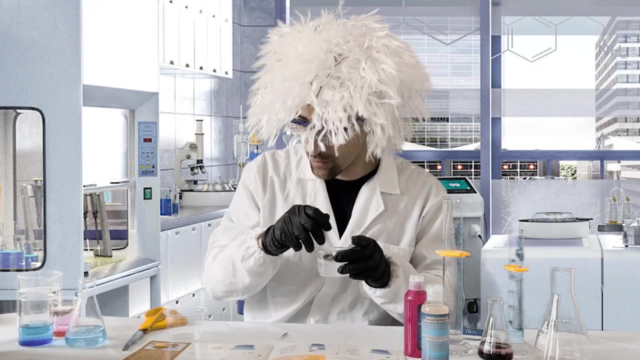 will react with the sodium alginate that we pour in. Now. what's going to happen is it's actually going to create calcium alginate, And so the substance itself, the material, is going to feel, instead of very liquidy, it's going to feel more viscous, like gooey, And that's because the gel 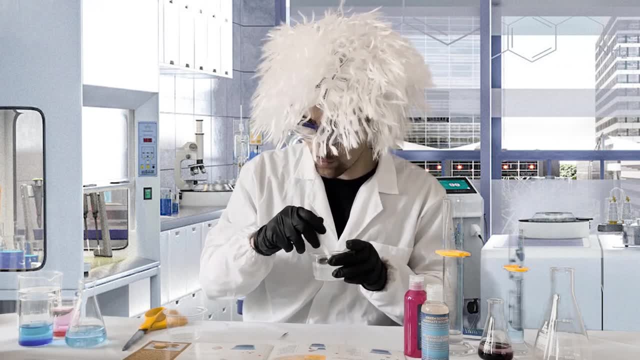 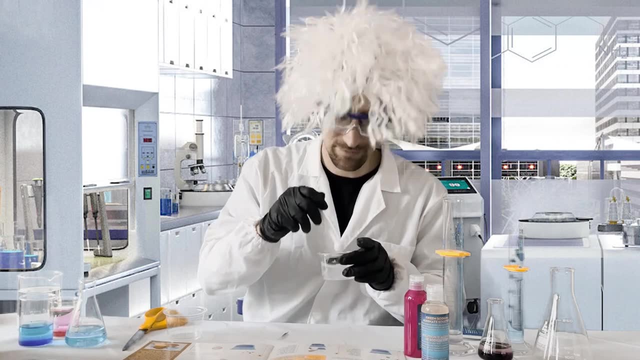 wraps around water droplets. So it's going to form these soft beads, or the worm eggs as we like to call them, And the longer the beads soak in the calcium chloride, the more calcium from this powder is going to seep into them, and the firmer 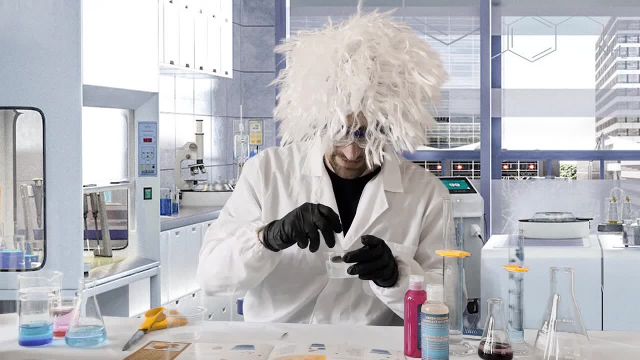 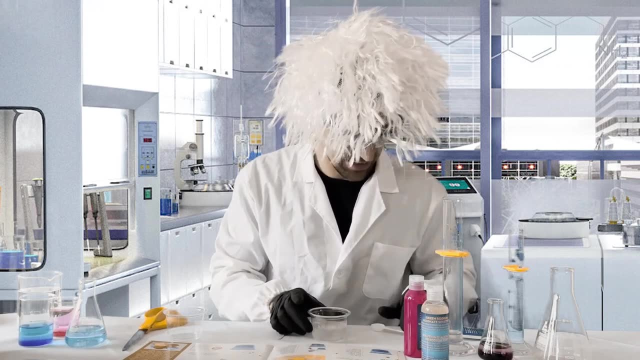 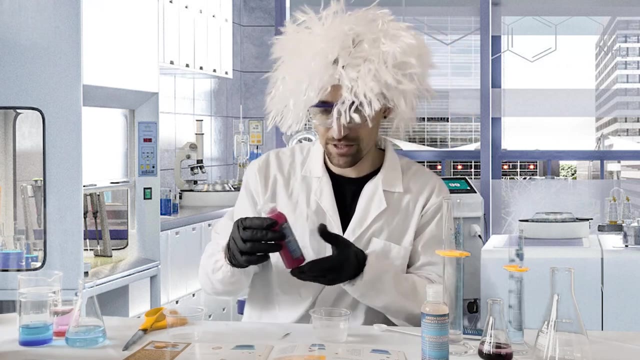 they're going to feel. So this looks about good. I've stirred it pretty well here. We're going to take now this half a cup of room temperature water that I mixed in a small spoon of my calcium chloride powder, And I'm going to open up carefully this color changing sodium alginate. 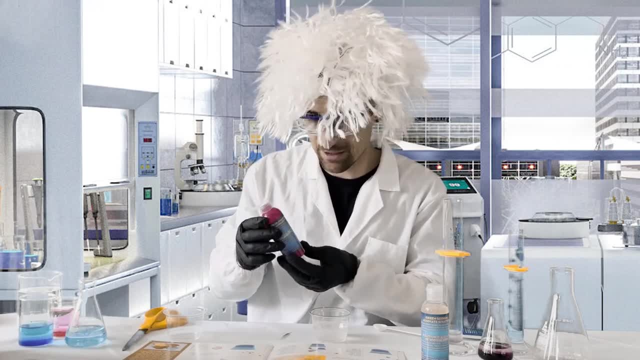 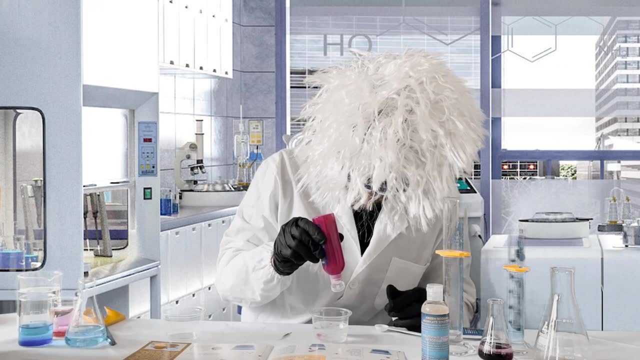 alginate solution, which, from the amazing worms chemistry kit, you could think of it as your red or pink solution. so just carefully, i'm going to start putting a few drops in here. i don't want to push too much, we don't want to stream, we want it to really come out as drops, and so you might. 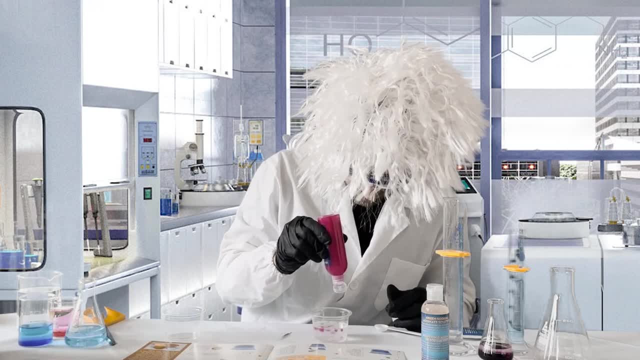 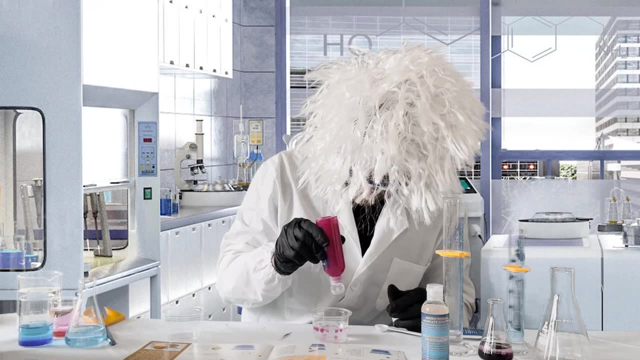 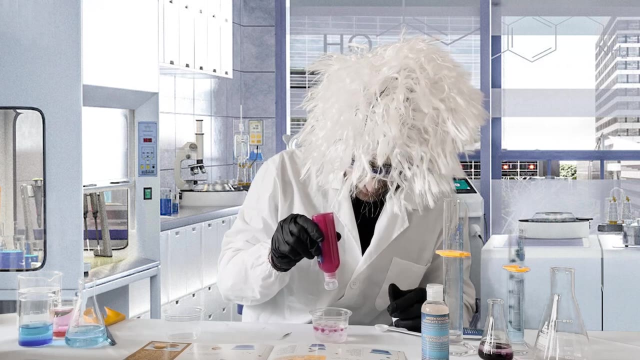 see some difference in the size of your drops. but just carefully put a couple of drops in here into this liquid and i can already see i have some very nice looking worm eggs forming here in my liquid solution, that calcium chloride liquid solution with the room temperature water. 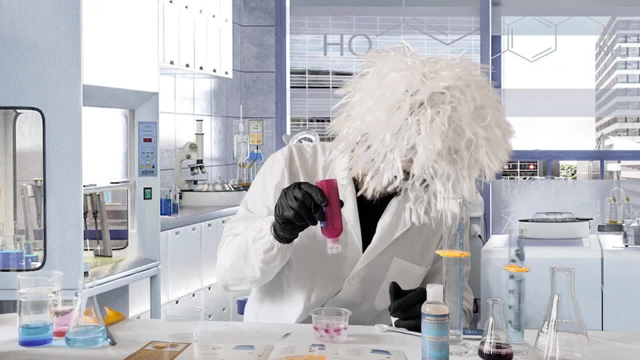 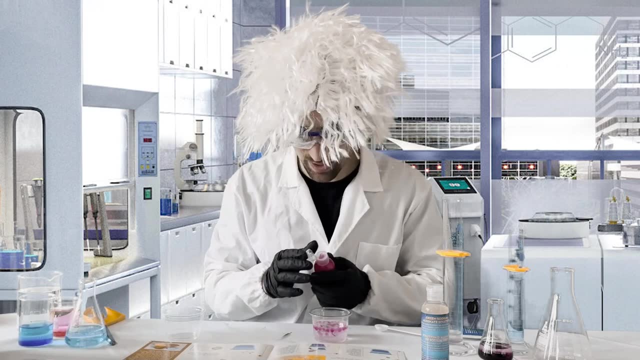 and so you could see, i'm just dropping very carefully, one drop at a time, one drop at a time, but that is forming these tiny little pink and red worm eggs, and so while that is going to be in the solution, and so, while that is going to be in the solution, 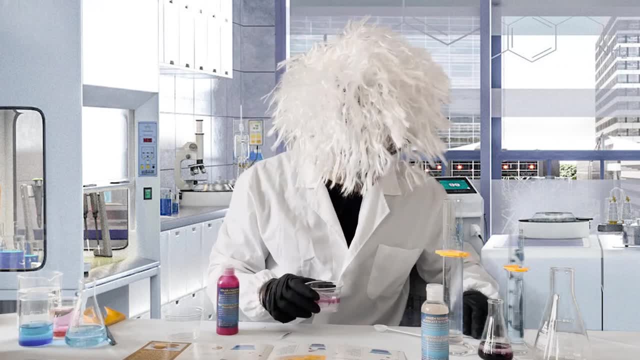 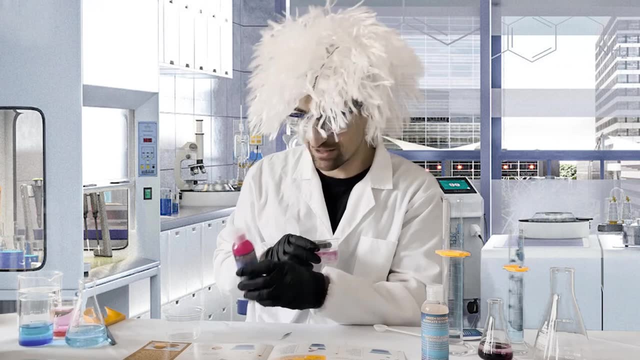 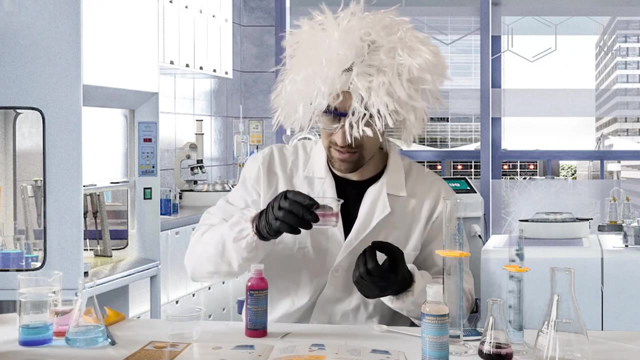 and so, while that is going to be in the solution, as highlighted, these two chemicals are coming together, this calcium chloride powder that we put in the water, as well as our, our color changing sodium alginate solution, and that's forming, as we've highlighted, calcium alginate, which is a kind of that new material with that different. 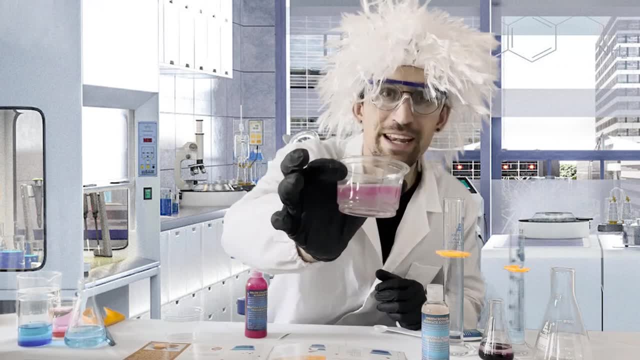 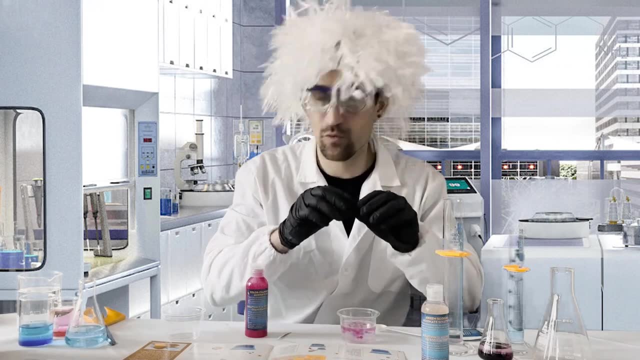 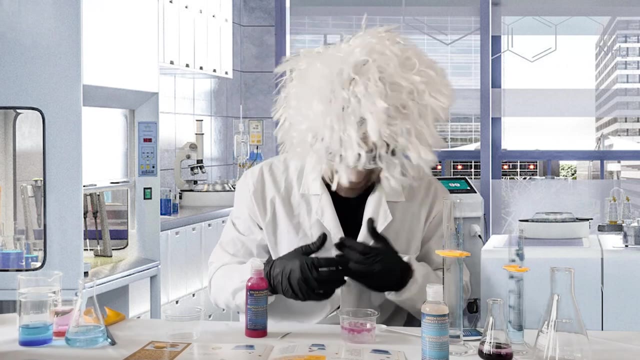 texture, and so we can see we have quite a few worm eggs in here and so we can let it sit, become a little more form form as it takes in a bit more of that calcium chloride seeping in and the calcium seeking into that gel making it firmer and firmer over time. or you can just head right in there into that water. 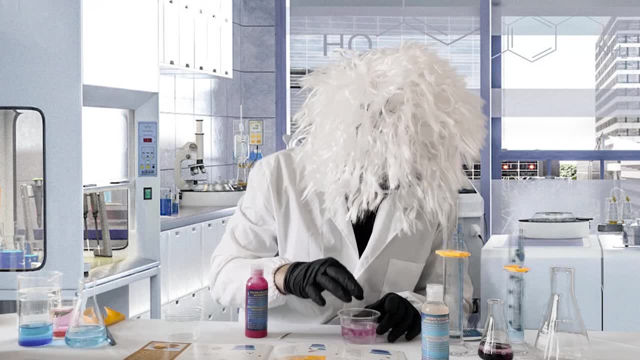 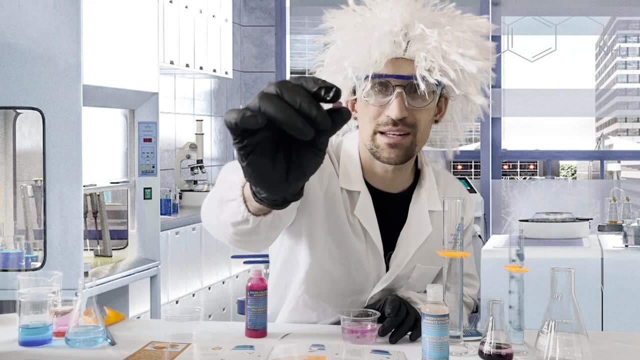 and you could try to pick out one of your little eggs. and so you could see, here i have got myself a little worm egg. it's very squishy, it's uh, i might drop it here, but it is quite an interesting texture. i can also squeeze it in. oh, there you go, it pops out a little bit and then you can see that. 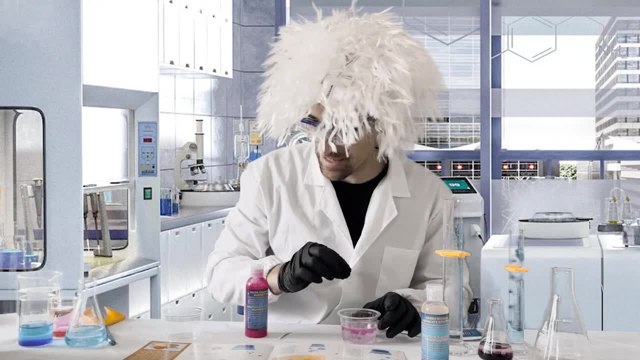 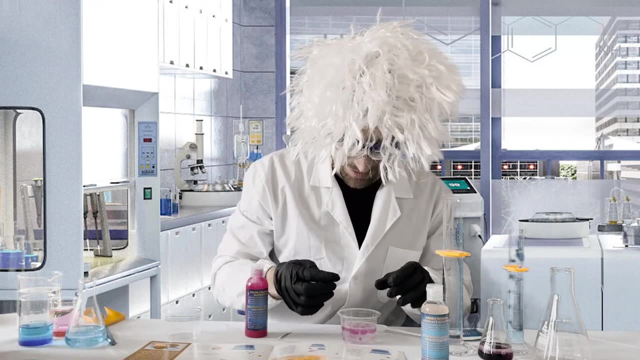 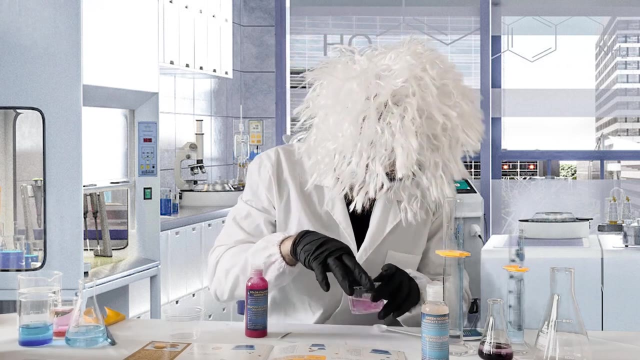 pops. it pops like that little gel sack that it is, and that's because, again, the gel is wrapping around. the water droplets is what's happening, and so why don't we now? we can play with this as we'd like- wash your hands after, of course- but we're going to keep one of these eggs for our next. 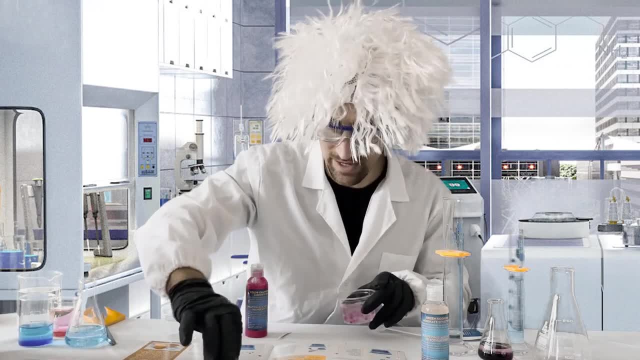 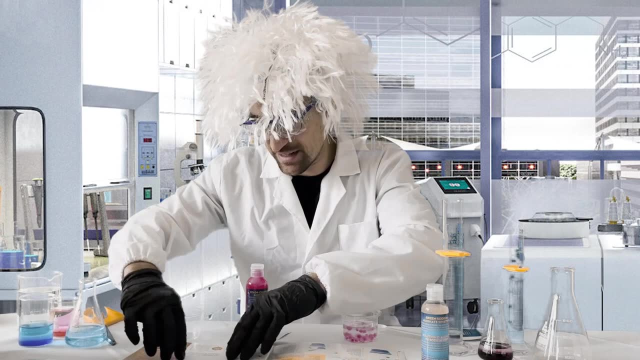 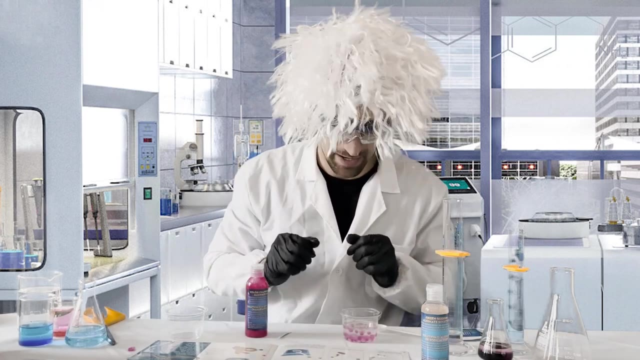 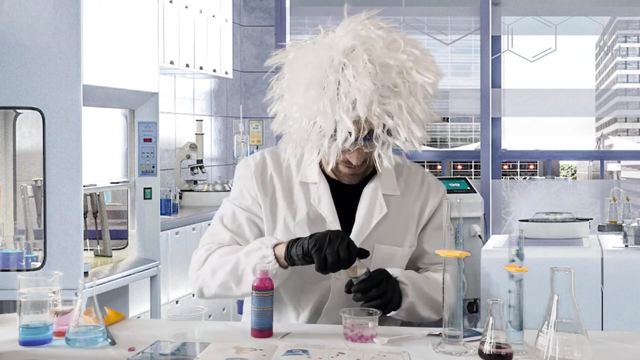 experiment. so i'm pulling out one egg here, i'm just going to leave it on. this experiment card is going to involve getting our kind of master green giant worm egg, and to do that we're going to go back to the measuring spoon. we're going to now fill it in with the green sodium alginate. 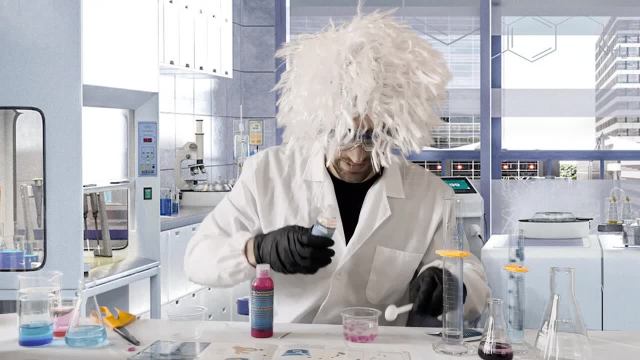 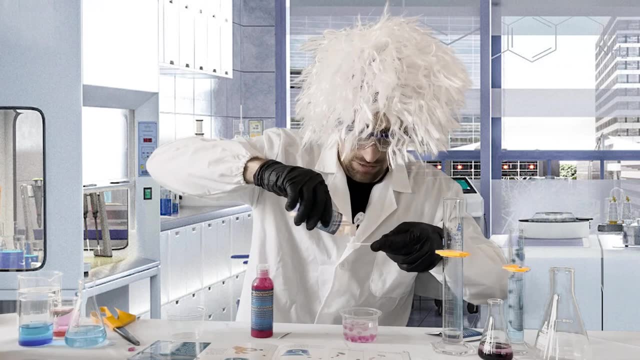 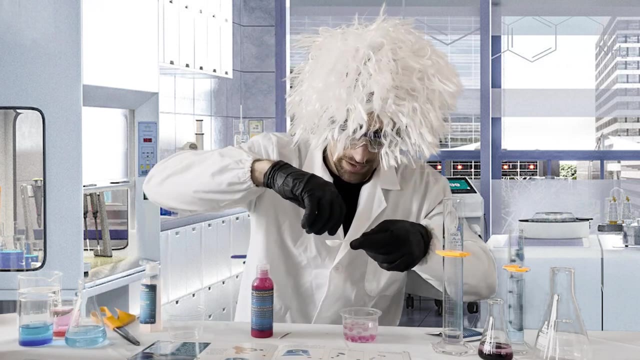 now, what we're going to do is we're going to pour this into our measuring- large measuring- cup, and we want to fill it up all the way, almost to the top. we're then going to take one- or even, if you want to do two, you can drop more than one in of our 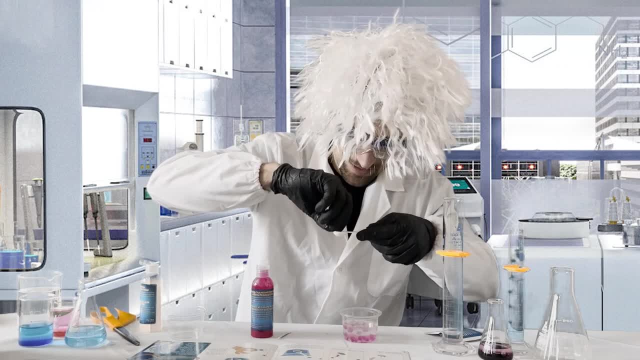 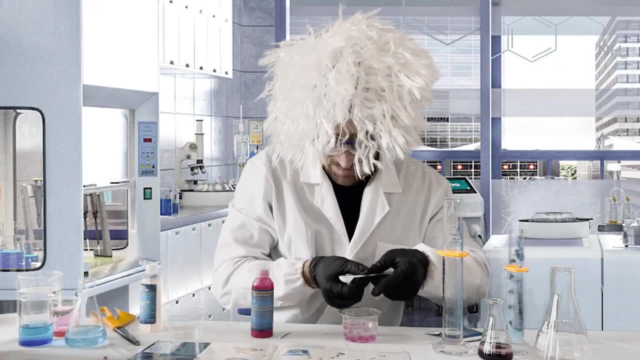 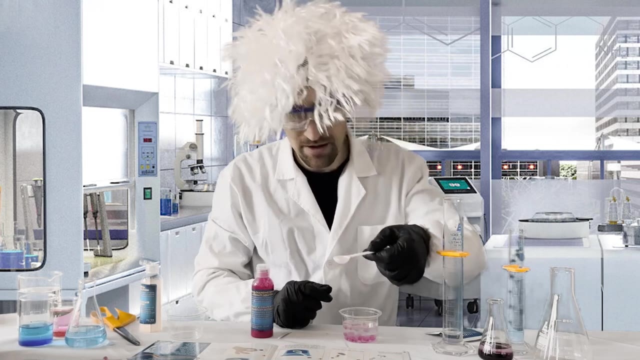 little pink worm eggs that we had previously created, and just go ahead and drop it into that large measuring cup side, and so you could move it around a little bit, let it sink down a little bit. but what we have now is this large spoon from our measuring kit. 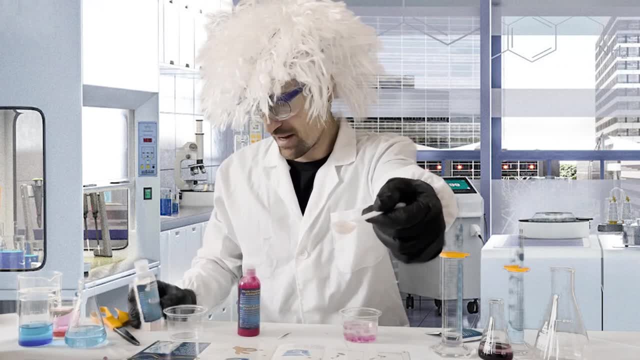 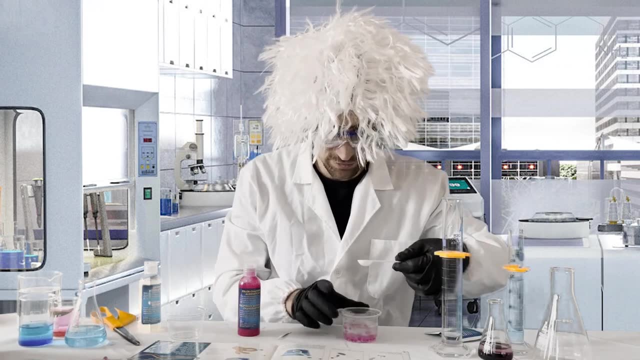 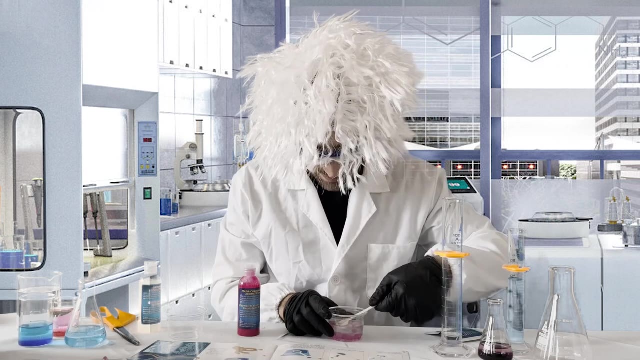 it has our worm egg that we created in our last experiment, and it's filled with this green sodium alginate solution. what we're going to do, then, is we're going to slowly submerge this egg with the green sodium alginate into the cold water, just slowly submerging it. 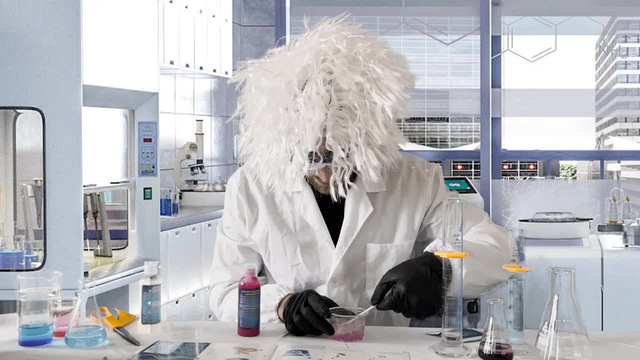 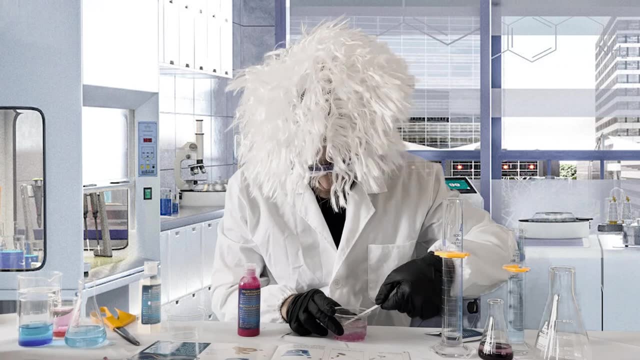 slowly, slowly, slowly submerging it. we're going to hold it steady for about 10 seconds here. if we can hold it steady for about 10 seconds here, if we can hold it steady for about 10 seconds here, if we can, and you'll notice that the giant egg should start solidifying. 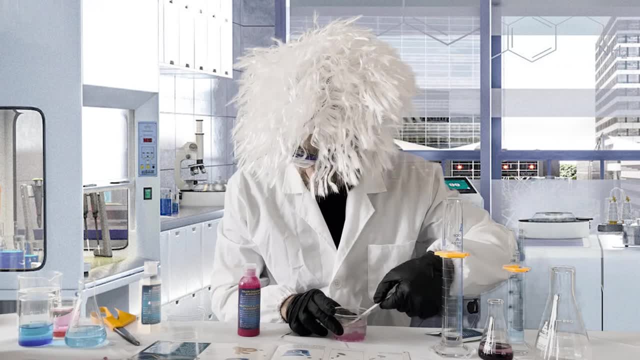 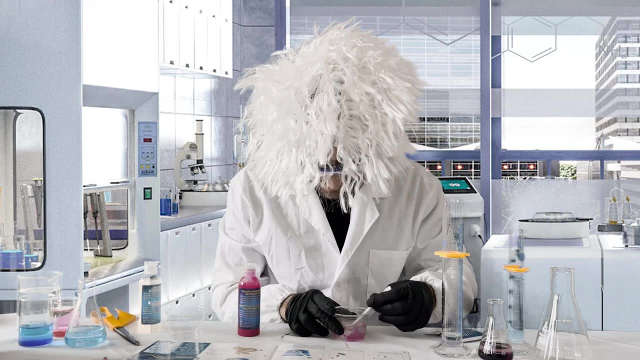 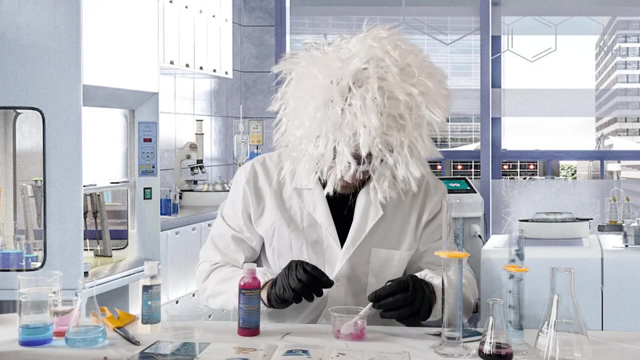 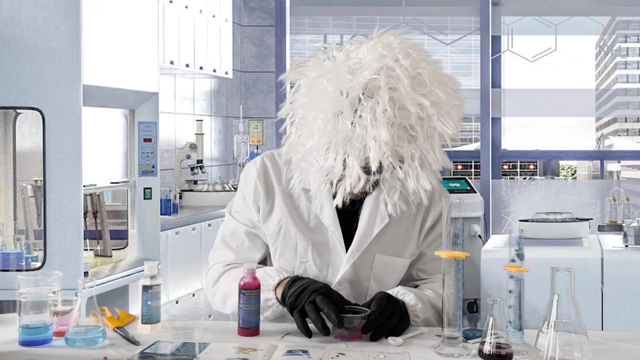 around our smaller egg. and now, if we gently, gently, gently start shaking the spoon, we can see and feel that giant egg breaking its connection and breaking free now, just like that. i can see i have my green egg floating here with the pink, and so i'm gonna go and i'm gonna fish this out and it might be easier for you. 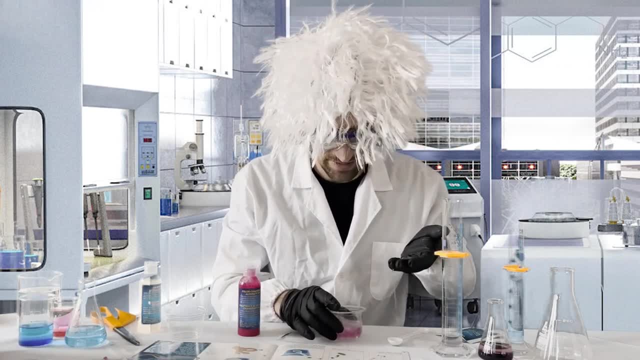 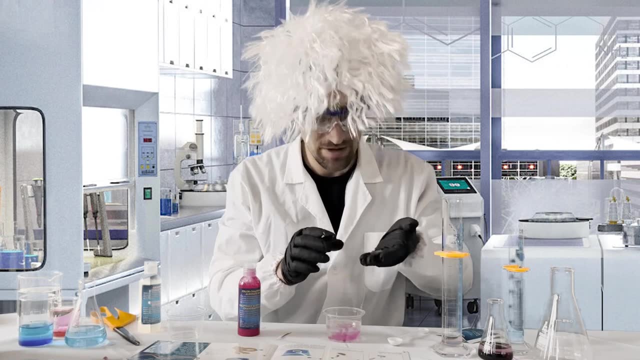 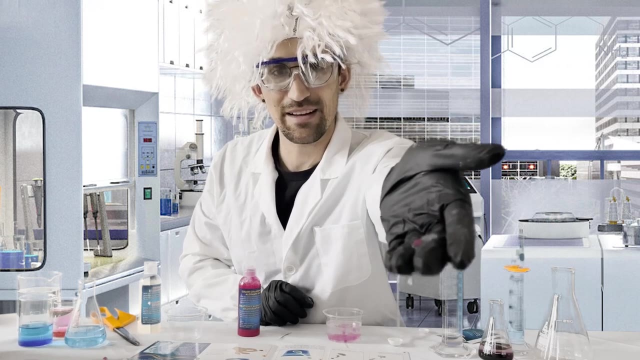 if you'd like to, uh, prior to jumping into this experiment, fish all of your other pink worm eggs out and just start with that water. that way it's easier to fish it out, but if not, it's still very easy to do. you can see, here i have this green goo mega egg and i have inside it. 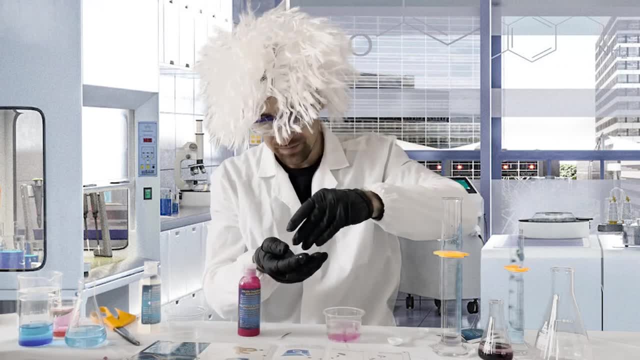 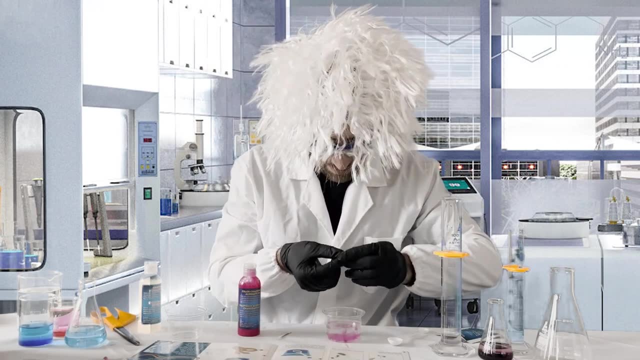 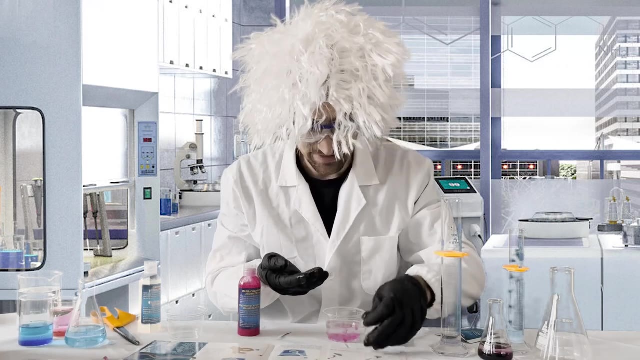 my pink egg. and so quite an exciting experiment, quite interesting to do, and once again we can pop this and we can get rid of that egg and pull out our pink worm egg from that green egg and so that material itself again is going to feel kind of like jelly, it's going to feel gooey. 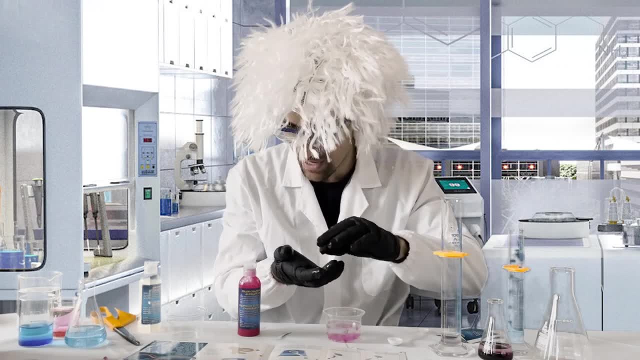 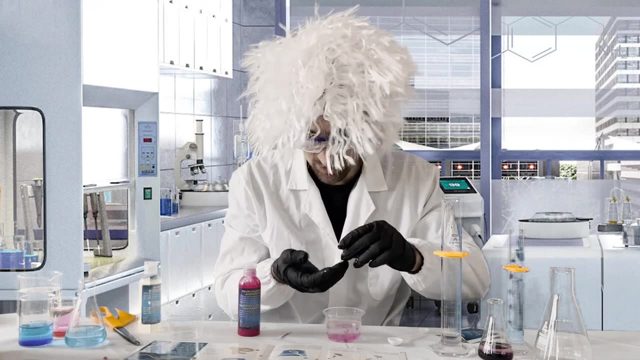 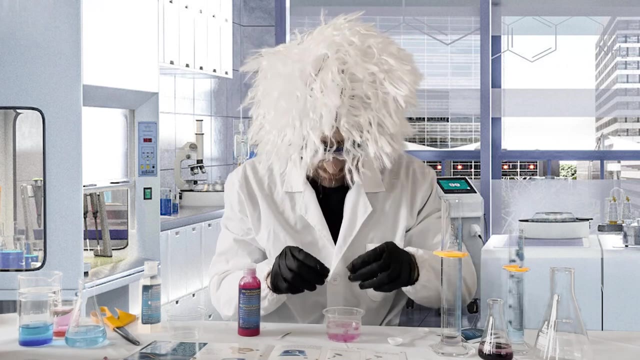 and, at the end of the day, it's because this sodium alginate is actually extracted from brown seaweed or kelp, and so that material, the alginate, is actually also used in a number of things: to thicken puddings, jams and even the chewing gum you might be eating, and so quite a fun experiment that we did today. 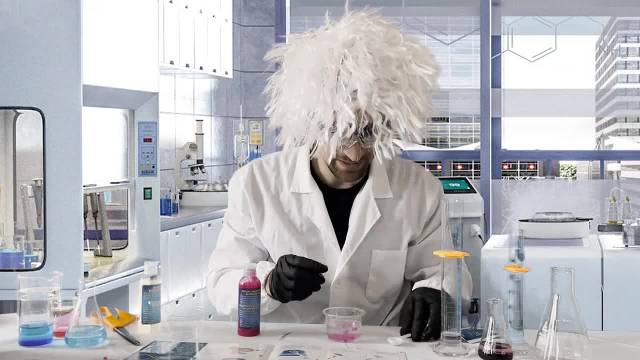 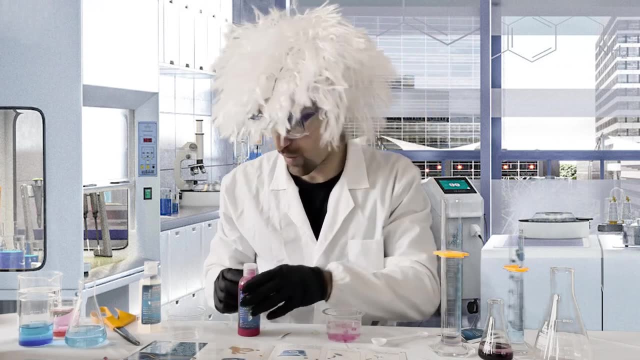 we've created a number of little pink worm eggs. we created a big worm egg in terms of a green worm egg, and feel free to play around with that as you'd like, as there's quite a lot of material for you to use. you can repeat that and make a few of these big worm eggs. try to get one, two.